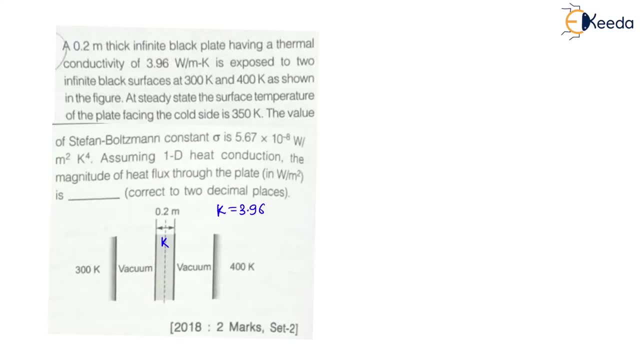 Therefore this thermal conductivity K value is 3.96 Watt per meter Kelvin. Now it is exposed to 2 infinite black surfaces at 300 Kelvin and 400 Kelvin. Now this 300 Kelvin surface is infinite black surface and this 400 and this 300 Kelvin also is infinite black surface. 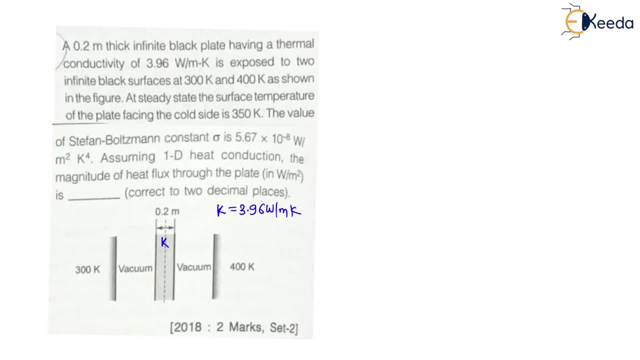 Right. So all are black surfaces, Right. Means we can say: all are black bodies, All are black bodies Right. This is very important. For black body emissivity is always equal to 1.. Means: emissivity of each and every surface is equal to 1.. 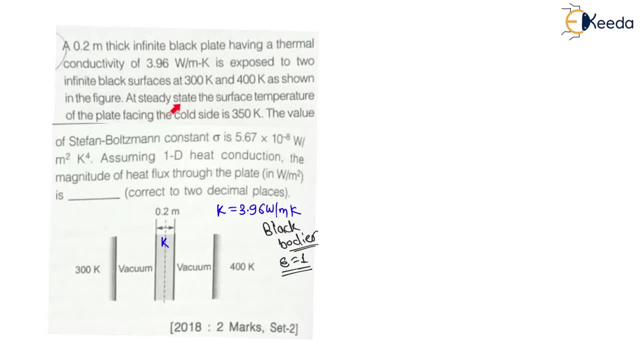 Then at steady state. the surface temperature of the plate facing the cold side is 350 Kelvin. Now here, between this 400 Kelvin and 300 Kelvin, This left side, that is 300 Kelvin, will be the cold side And the plate facing towards this cold side is at 350 Kelvin temperature. 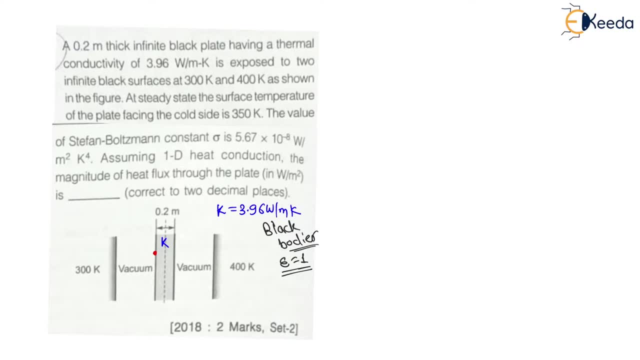 Therefore, my dear students here on this black plate, this temperature is 1.. Let us say here I will give the names of plates, Right. Let us say here this will be the plate at highest temperature, is plate number 1.. Let us say: this is the another side of the black plate. 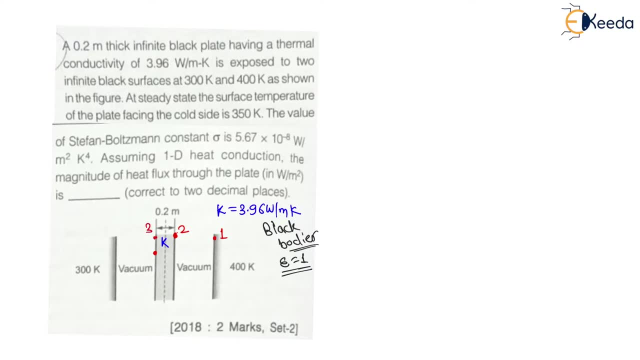 Here. this is the third side. Third, And this is the fourth plate, These are the four plates, Right? Therefore, we can say: T1 is equal to 400 Kelvin, T4 is equal to 300 Kelvin And T3 is given. 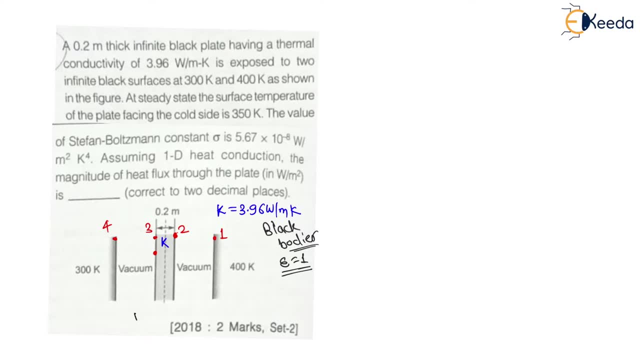 Right. So, my dear students here, value of T3 is given. We can say: T3 temperature of third plate is 350 Kelvin. It is 350 Kelvin. The value of Stefan-Bohlmann constant sigma is Now here. Stefan-Bohlmann constant sigma is given. 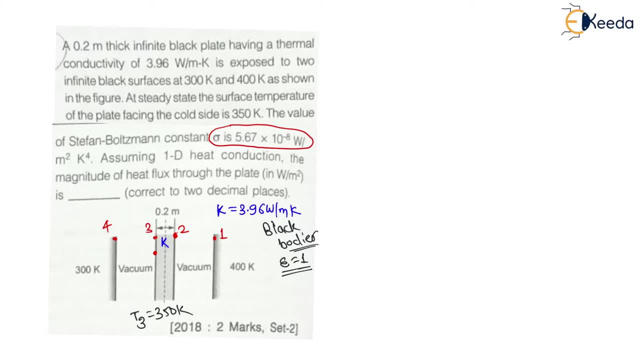 Which is 5.67 into 10 to the power minus 8. Watt per meter square Kelvin. It is a standard value of sigma. Assuming 1D heat conduction, The magnitude of heat flux through the plate in Watt per meter square is: 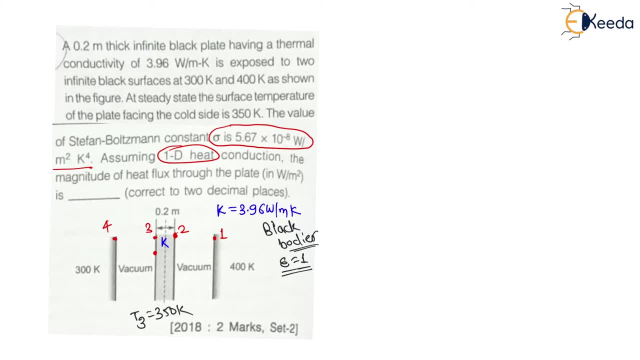 Now here they are mentioning it is a one directional heat transfer And the magnitude of heat flux through the plate Right. They are asking: what is the heat flux? Let us say Q. Heat flux is heat transfer rate per unit area, which is in Watt per meter square. 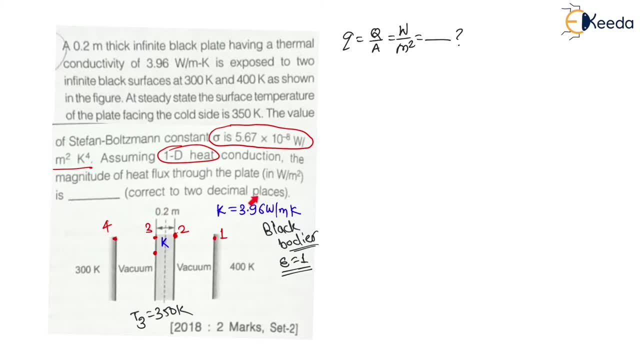 This value we have to find Right, Correct to the two decimal places. So let us solve this question Now. my dear students in question. they have mentioned that it is a 1D heat conduction, That is, 1D heat transfer as well as it is a steady state. 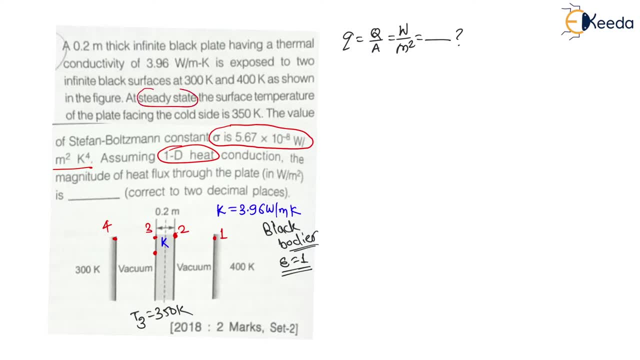 They have mentioned Right. This is a very important condition. 1D: steady state. Now, my dear students, for 1D there will be a heat transfer along one direction only, And for steady state, the temperature at each and every location will be same or constant. 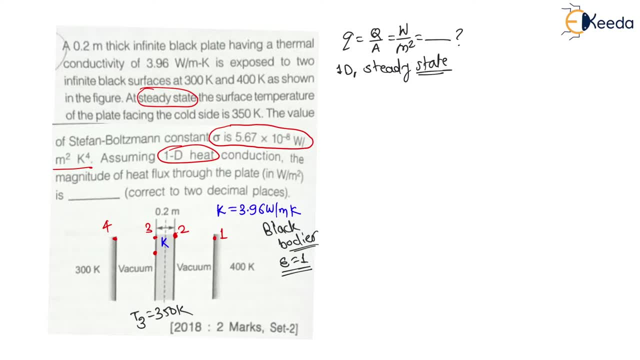 at that particular location. with respect to time, That is. steady state means temperature is not a function of time. With respect to time, the temperature of any location is not going to change. Means here. this: T1 will be always constant at any time. T2, T3 and T4 will be constant at their respective values at any time. 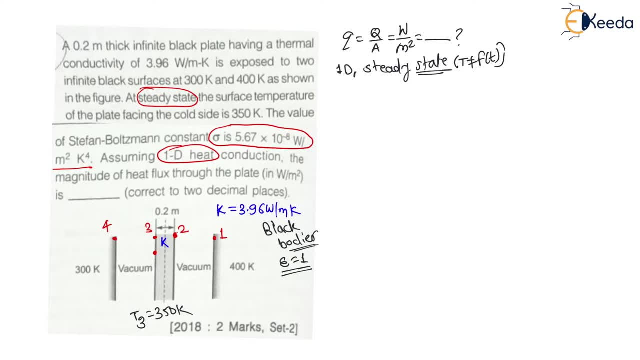 Right, This is called steady state And my dear students, for this 1D steady state, the heat transfer rate, that is, let us say, Q Heat transfer rate in Watt, is always constant at each and every location. At every location, heat transfer is always constant. 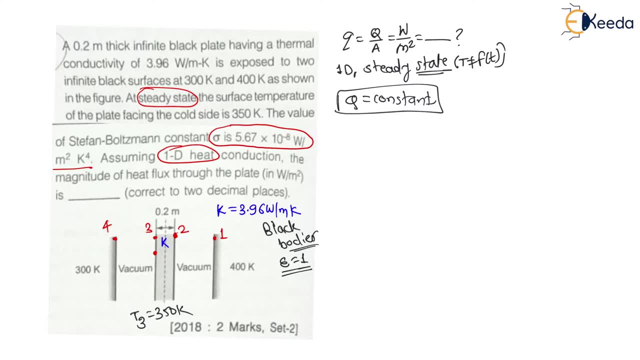 Right Now, my dear students, let us understand the mechanism of here: heat transfer Now from surface 1 to surface 2. there is perfect vacuum. Therefore there will be a radiation In vacuum. there is a radiation Means between 1 and 2. there will be a heat transfer by radiation. 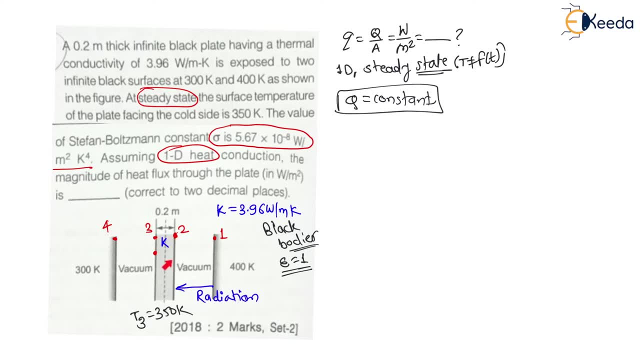 Now again, from 2 to 3 there is a black plate. Right It is a plate. Therefore, in solids there will be a conduction Means. my dear students, between 2 to 3 there will be a conduction heat transfer Right. 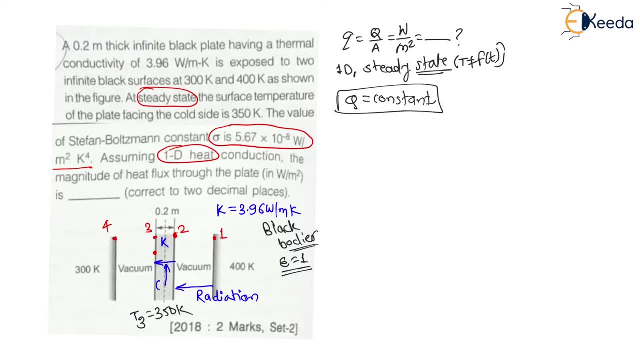 Therefore, from 2 to 3 the mechanism of heat transfer will be conduction. here It will be a conduction Right. Then, from 3 to 4, again, there is a perfect vacuum. Therefore, between 3 to 4, again, there will be a radiation heat transfer. 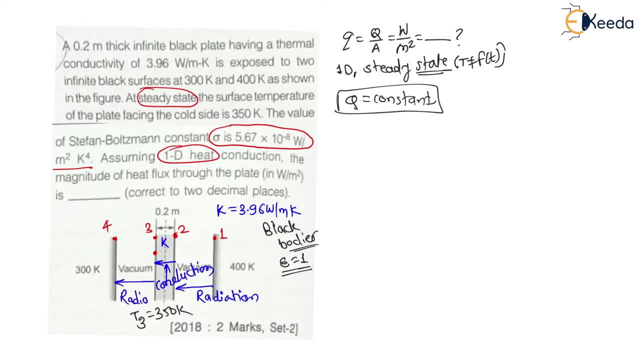 Right 3 to 4, there will be a radiation heat transfer Right And, my dear students Here, the heat transfer between 1 to 2 is equal to heat transfer rate, is equal to heat transfer between 2 to 3 is equal to heat transfer between 3 to 4. now the question. 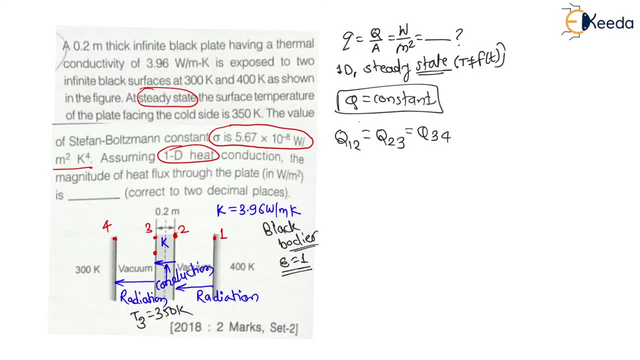 is to find heat flux, that is heat transfer rate per unit area. now here i can use any one formula now, as temperature t3 is given as well as t4 is given means temperature between 3 to 4. this temperature difference we have available right, so we can use. that is heat transfer between 3 to 4. 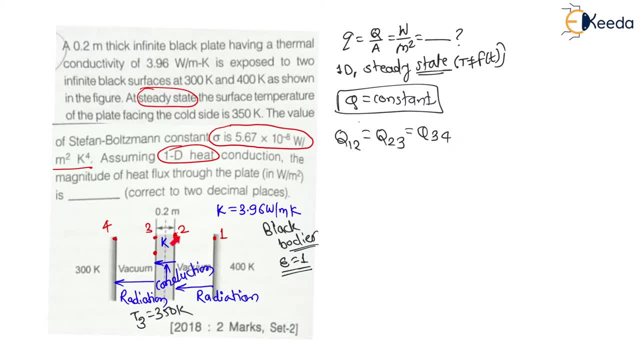 for calculation of heat flux right, because if i use 1 to 2, here t1 is known, but t2 is unknown. if i use 2 to 3, then t2 is unknown, but t3 is known. but for 3 to 4 both temperatures are known. 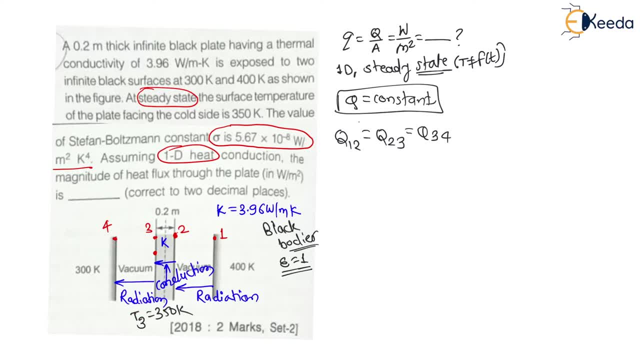 and between 3 to 4 there is a heat transfer by radiation. therefore, my dear students, here we can write: the heat transfer between 3 to 4 is nothing but heat transfer by radiation, heat transfer by radiation between 3 and 4. therefore, this heat transfer between 3 to 4, the radiation heat transfer, is given as sigma, that is stephen. 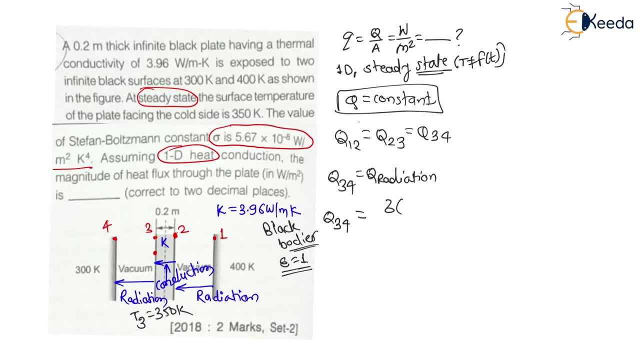 bollman constant. this is a stephen bollman constant as it is 3 to 4. it is t3 power 4 minus t4 power 4 divided by 1 minus emissivity 3. divided by area 3: emissivity 3 plus 1 upon area 3 f 3 to 4 plus. 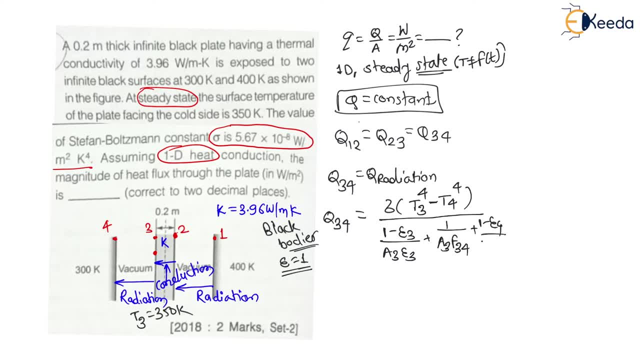 1 minus emissivity 4 divided by area 4, emissivity 4: right. this formula we have seen, that is radiation heat transfer between the infinite plates right, and here they have given infinite black plates right. in this question they have mentioned that infinite black plates right, as it is black plate for black plate or for black. 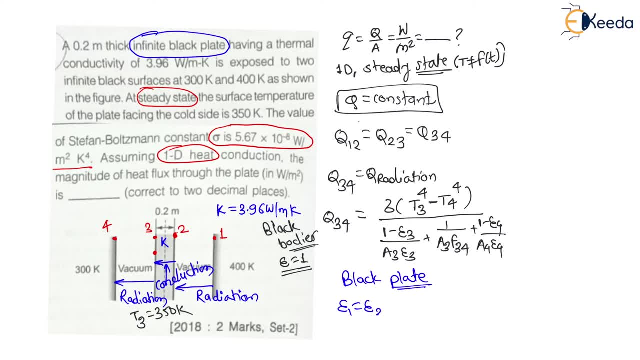 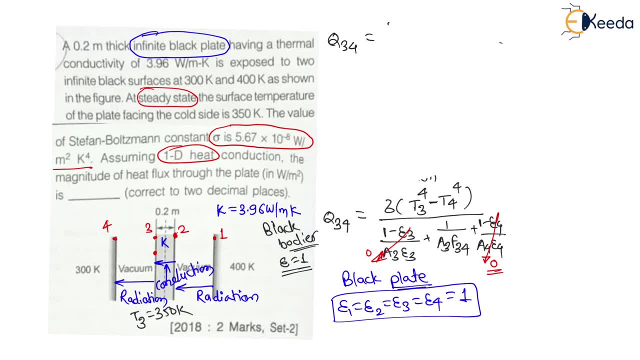 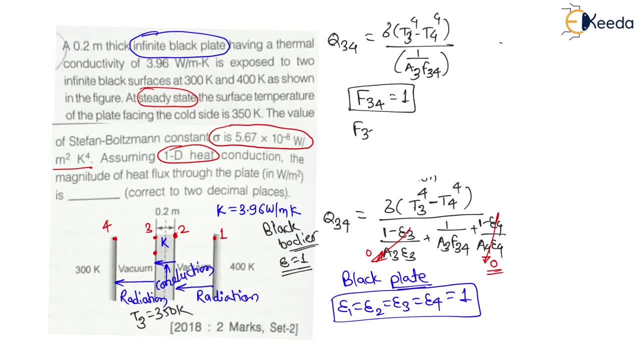